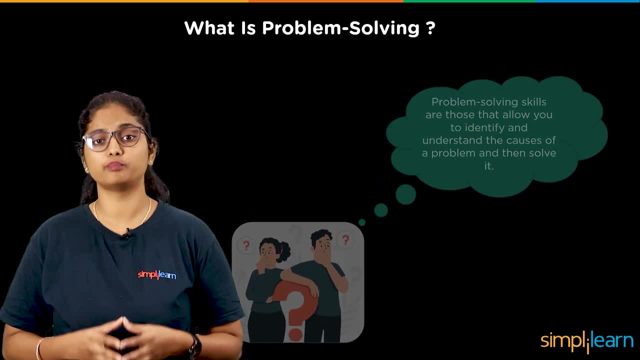 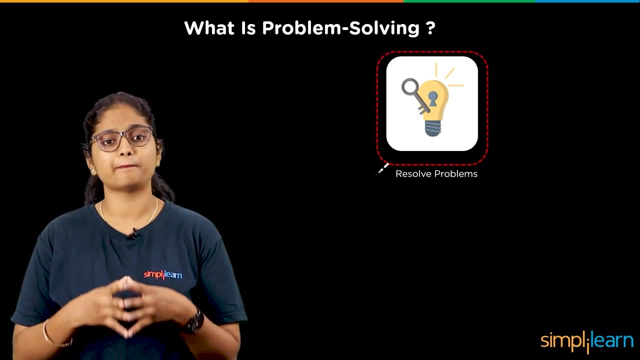 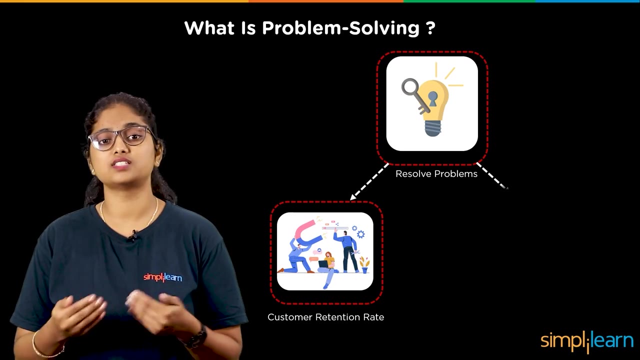 An effective problem-solving is the ability to make an employee both a self-starter and a good team member. For example, it might resolve the problems that might impact the entire company, such as decrease in the customer rate retention, or some problems that might impact you, such as. 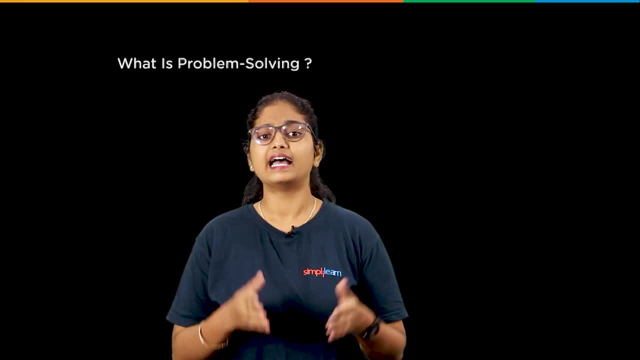 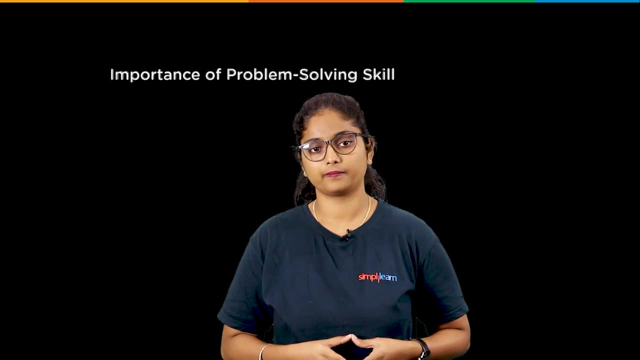 decision-making, critical thinking, etc. After getting a brief about problem-solving, now let us understand why it is important in our personal and professional life. The problem-solving is a skill for those which will help to identify and understand the problem-solving. The problems you might experience at the workplace are endless, So you should be capable of finding. 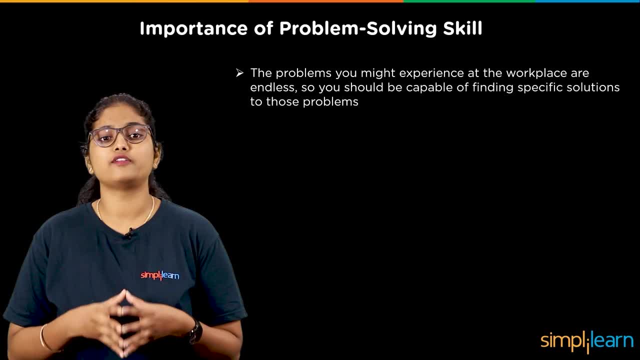 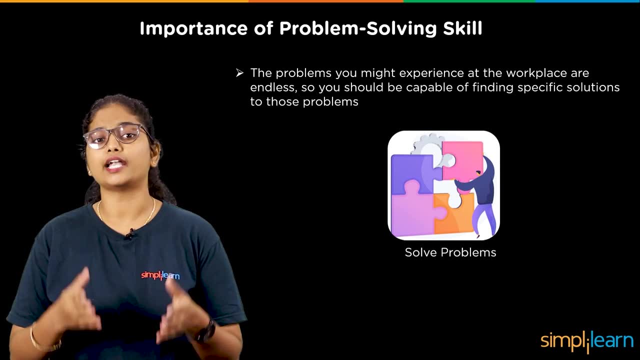 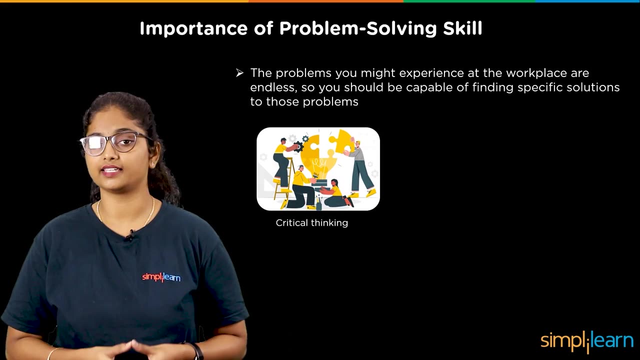 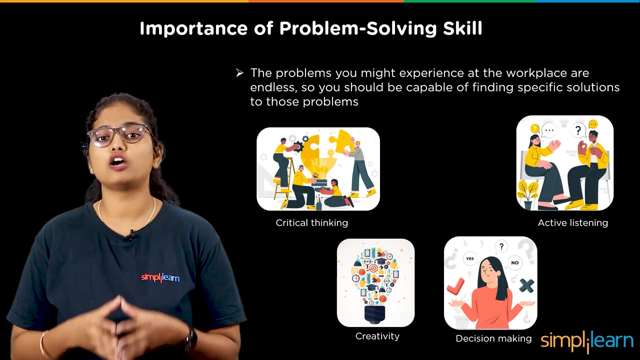 the specific solutions for those problems. Problem-solving skills are important for several reasons. For one, they can help you in better understanding and solve the problem that you encounter in your everyday life and workplace. Also, it enhances some of your soft skills, such as critical thinking, active listening, creativity, decision-making and many more. By now, I am sure, 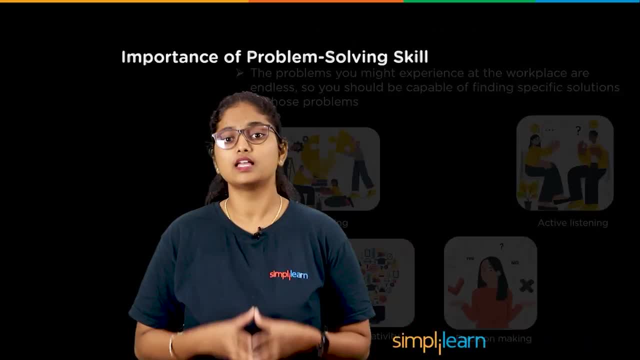 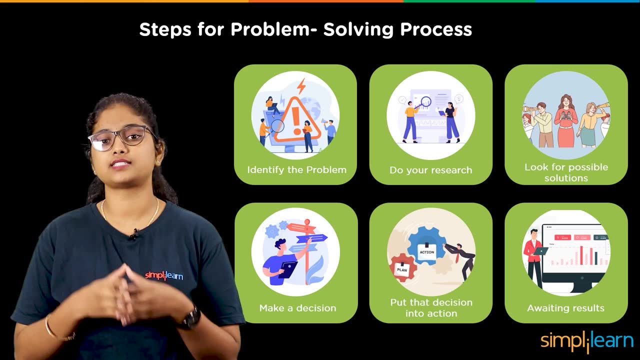 you have got some idea about the problem-solving and its importance. Now let us go through the steps that comes under the problem-solving process. Problem-solving requires a systematic, step-by-step approach to a challenge. Here are some basic tips of problem-solving that you can. 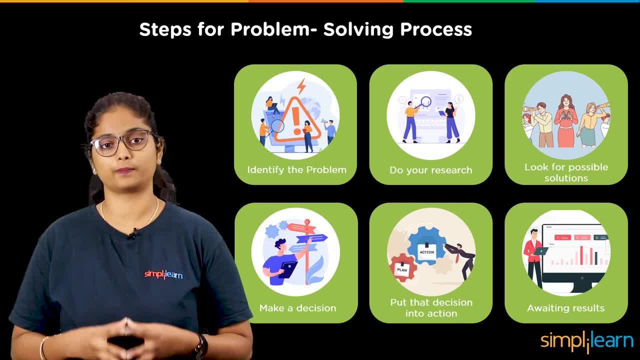 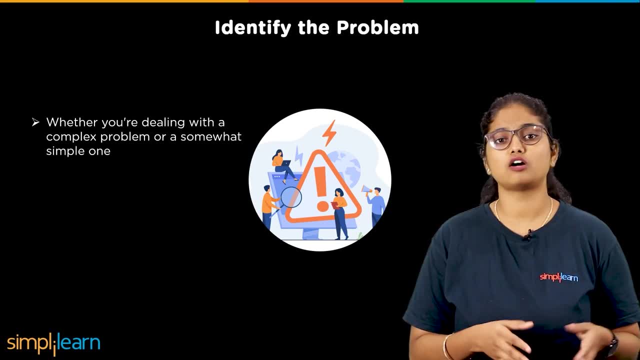 follow. when you are approaching a problem in your personal life or a workplace, The first step is to identify the problem. When you are dealing with a problem, which can be a complex or somewhat simple one, you must clearly understand what you are trying to solve. You must clearly understand what you are trying to solve. 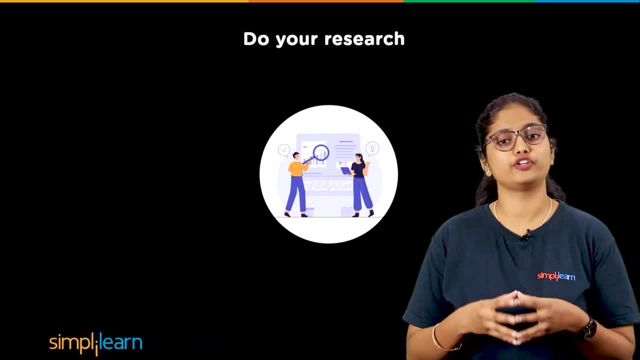 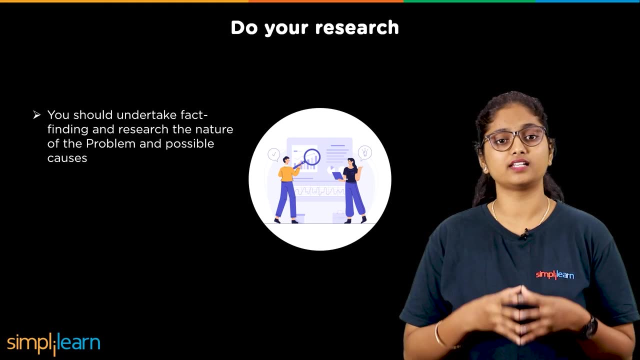 The next step is to do your research. Once you have a clear idea about the problem you are solving, you should undertake a fact-finding and a research of the nature of the problem and the possible causes. This research process might include looking into reasons for similar. 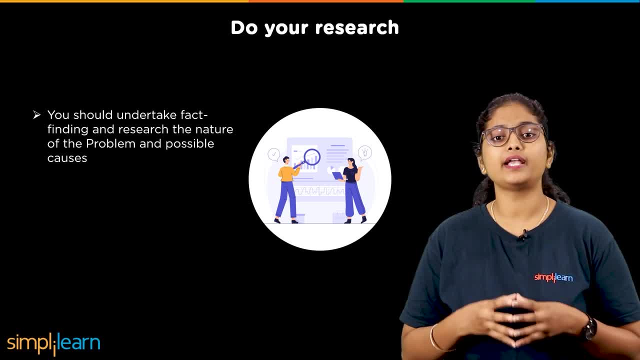 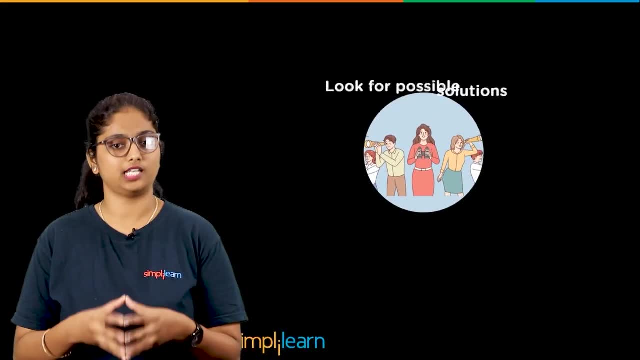 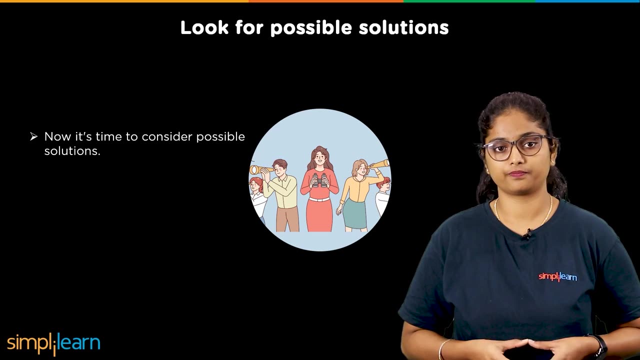 problems that have been resolved in the past, or it might require planning or interview questions to ask for those who are involved in the issue. The third step is to look for the possible solutions. After doing all the required research about the problem, now it's time to consider the possible solutions. 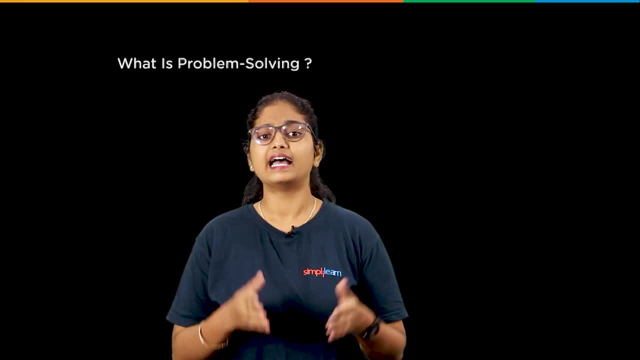 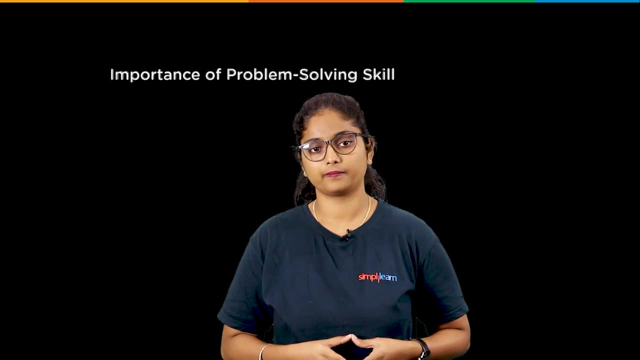 decision-making, critical thinking, etc. After getting a brief about problem-solving, now let us understand why it is important in our personal and professional life. The problem-solving is a skill for those which will help to identify and understand the problem-solving. The problems you might experience at the workplace are endless, So you should be capable of finding. 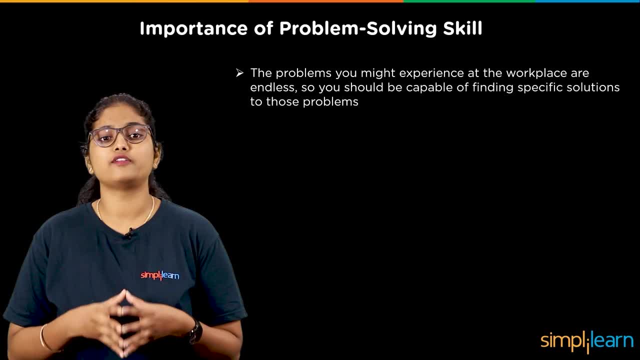 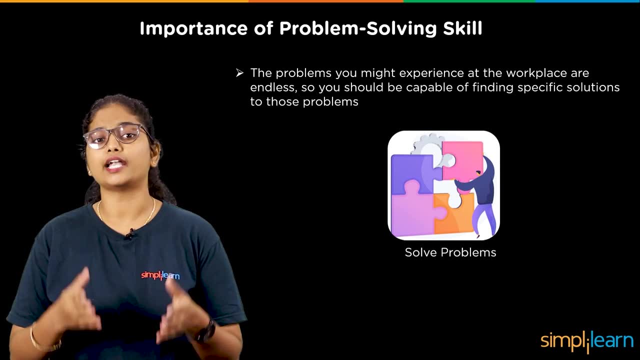 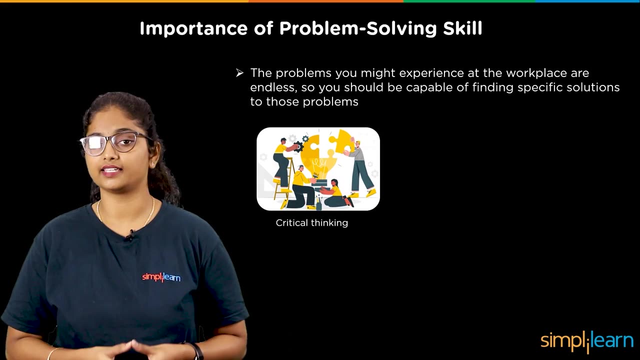 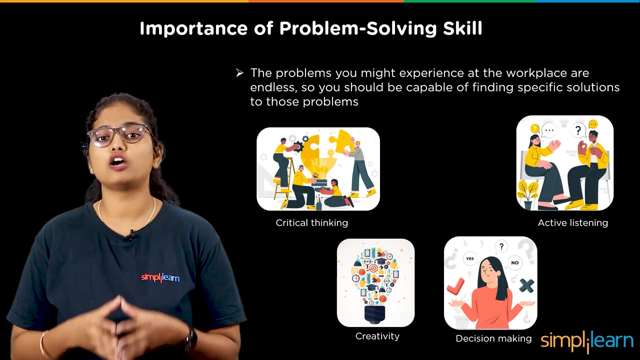 the specific solutions for those problems. Problem-solving skills are important for several reasons. For one, they can help you in better understanding and solve the problem that you encounter in your everyday life and workplace. Also, it enhances some of your soft skills, such as critical thinking, active listening, creativity, decision-making and many more. By now, I am sure, 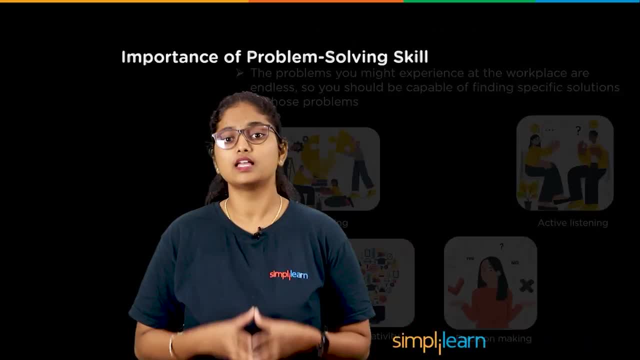 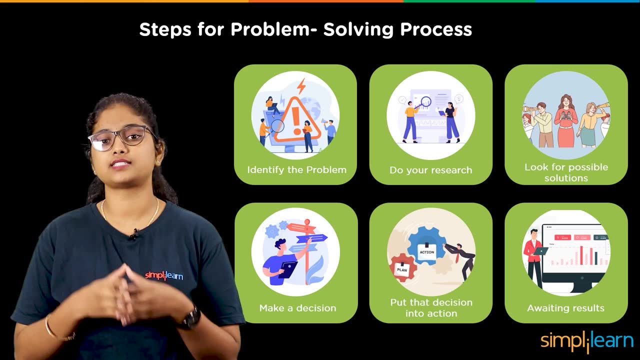 you have got some idea about the problem-solving and its importance. Now let us go through the steps that comes under the problem-solving process. Problem-solving requires a systematic, step-by-step approach to a challenge. Here are some basic tips of problem-solving that you can. 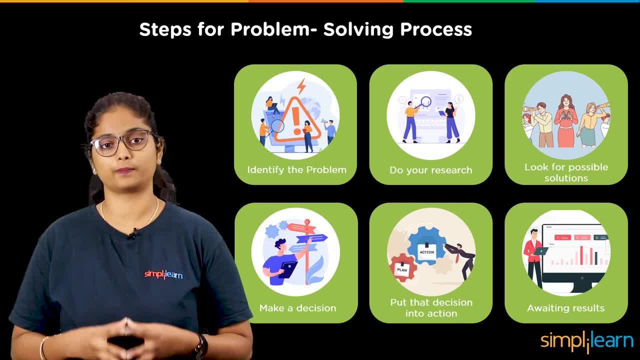 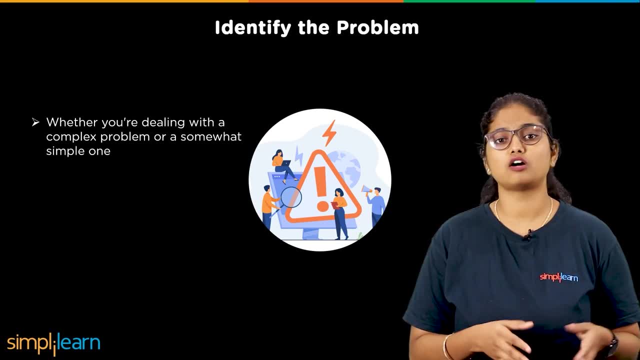 follow. when you are approaching a problem in your personal life or a workplace, The first step is to identify the problem. When you are dealing with a problem, which can be a complex or somewhat simple one, you must clearly understand what you are trying to solve. You must clearly understand what you are trying to solve. 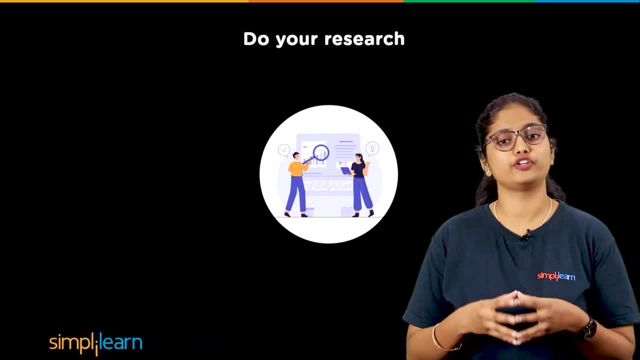 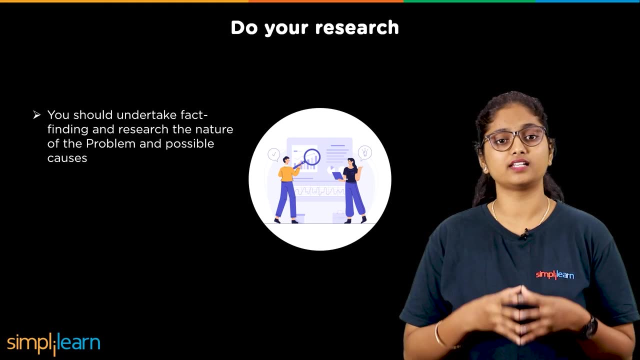 The next step is to do your research. Once you have a clear idea about the problem you are solving, you should undertake a fact-finding and a research of the nature of the problem and the possible causes. This research process might include looking into reasons for similar. 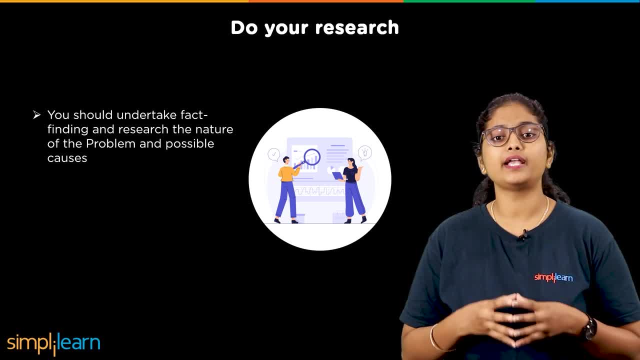 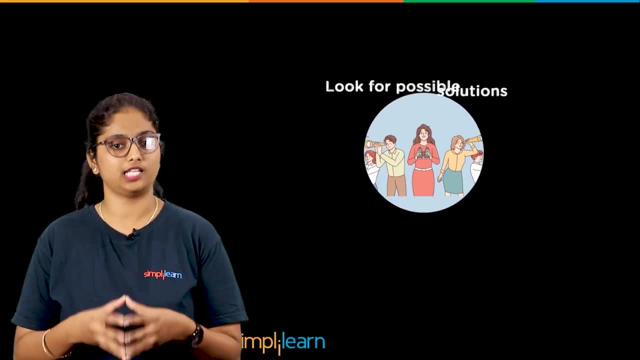 problems that have been resolved in the past, or it might require planning or interview questions to ask for those who are involved in the issue. The third step is to look for the possible solutions. After doing all the required research about the problem, now it's time to consider the possible solutions. 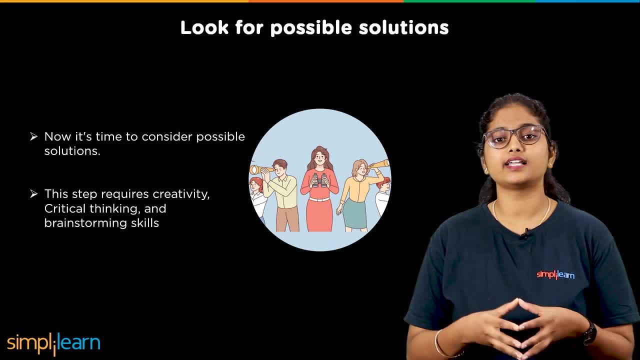 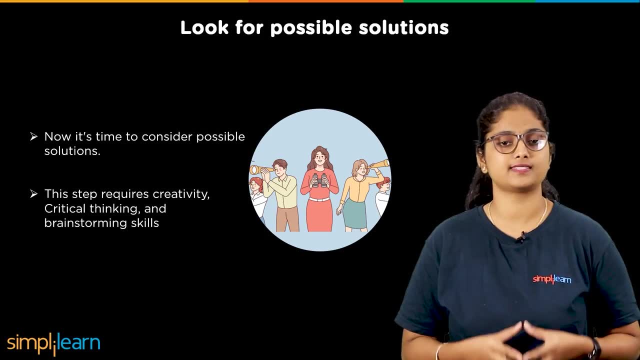 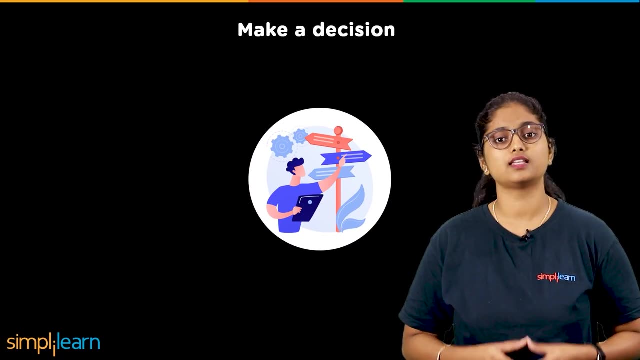 These steps require creativity, critical thinking and brainstorming skills to look for the possible solutions and also for the alternate solutions if the solution fails. The next step is to make a decision. Once you have all the list of possible solutions and the alternative solutions, it's time to narrow. 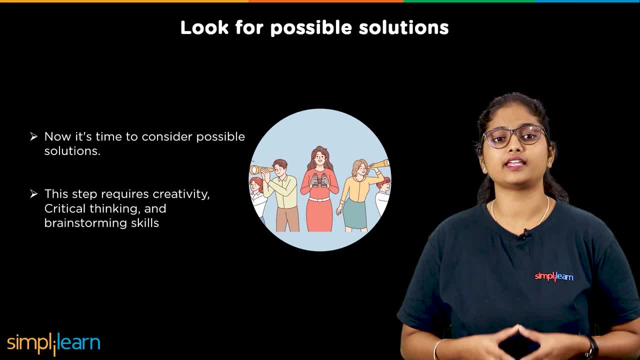 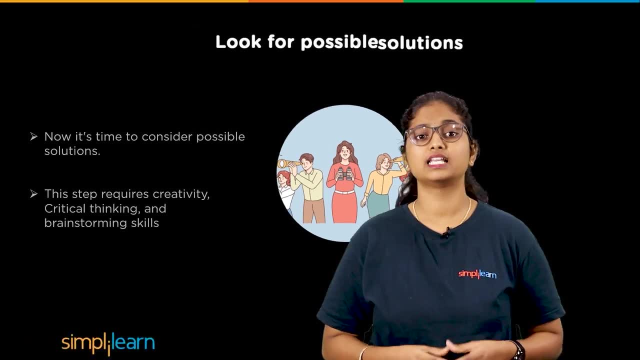 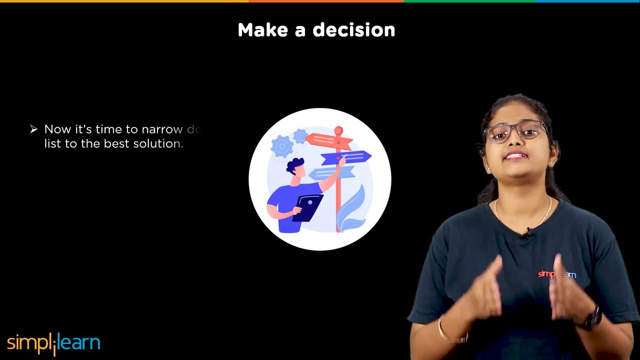 These steps require creativity, critical thinking and brainstorming skills to look for the possible solutions and also for the alternate solutions if the solution fails. The next step is to make a decision. Once you have all the list of possible solutions and the alternative solutions, it's time to narrow. 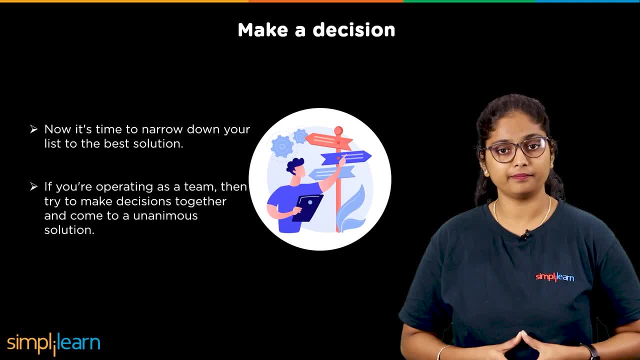 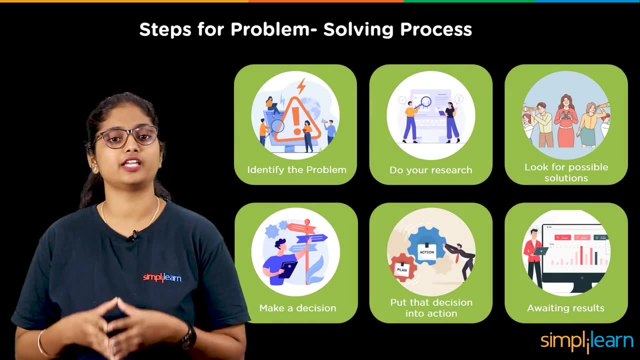 down your list into a best solution. If you are operating in a team, try to make a decision, to gather and come to an unanimous solution. The fifth step is to put the decision into an action. Implementing your selected solution is in a planned and calculated way will avoid the action. 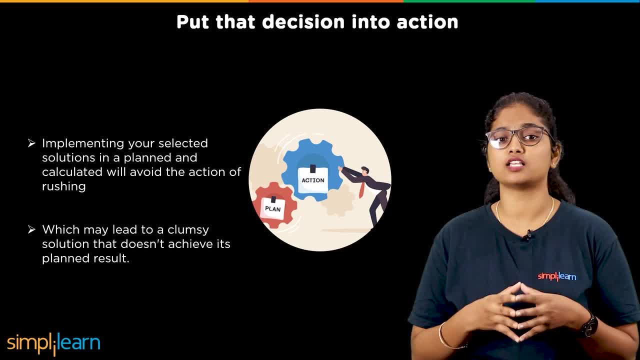 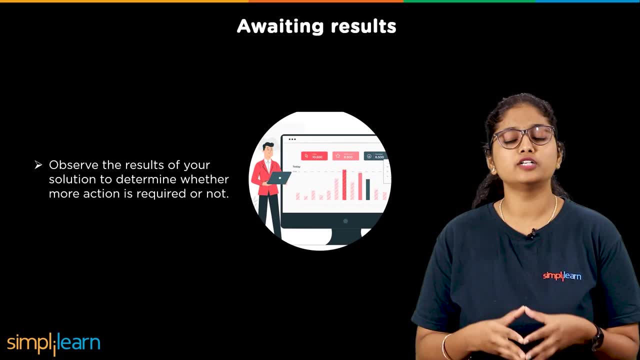 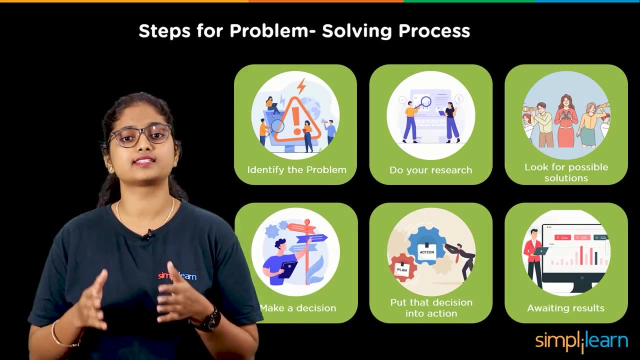 of rushing, which may also lead to a clumsy solution that does not achieve the planned result. And the last step is to awaiting for the results. Observe the results for your solution to determine whether the more action is required or not. Now let's see the skills or a. 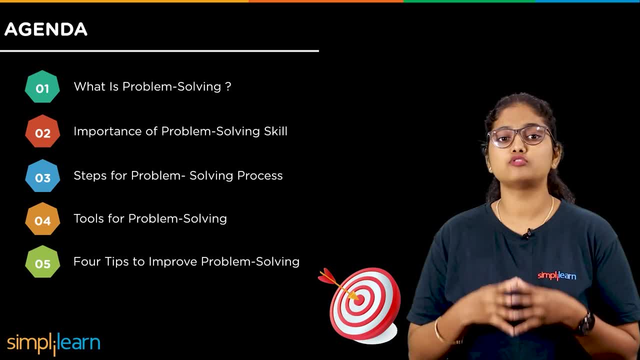 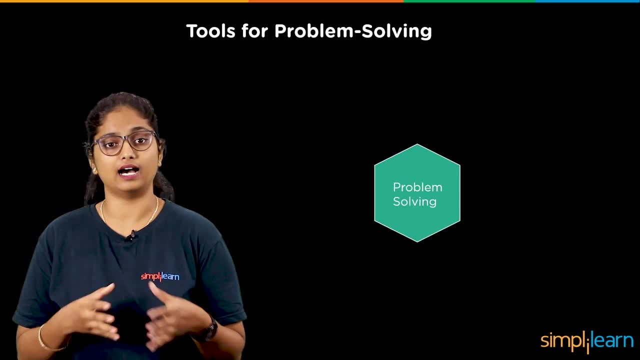 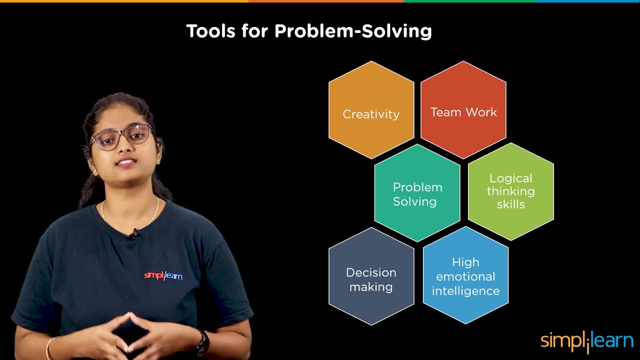 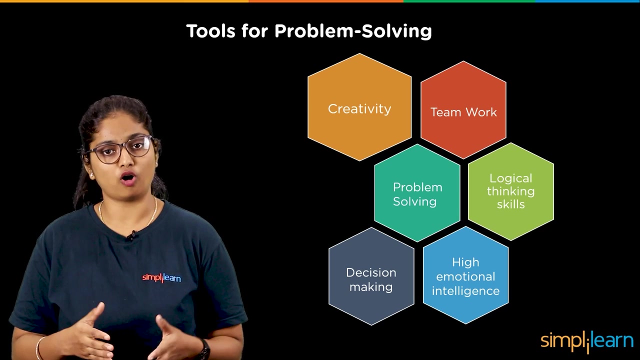 tools required for the problem solving. The best problem solver often have a few fundamental skills. The most important skills to draw upon when engaging a problem solving process are creativity, teamwork, logical thinking and high emotional intelligence and, at last, decision making. Let's see, one by one, Creativity: Creativity helps to think outside the box and reach out. 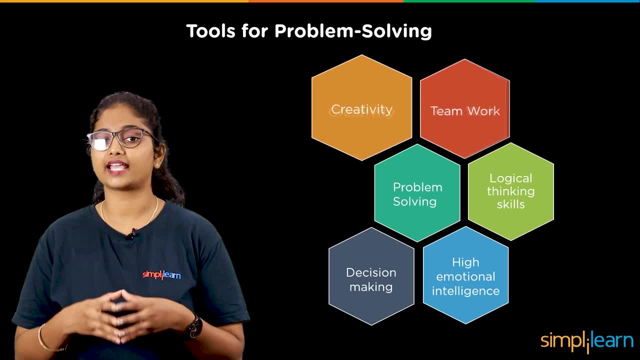 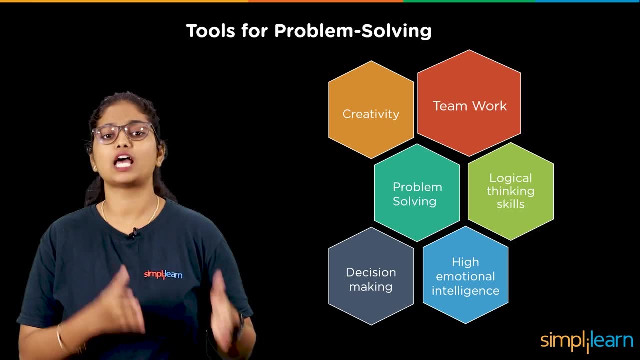 the new techniques and understand the problems. Next is a teamwork. Teamwork will help you address a group or a social problem which requires working in a team collaboratively and supportively. On the list, we have a logical thinking skills To analyze the 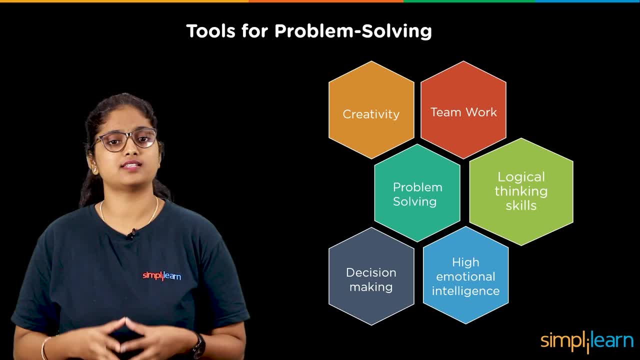 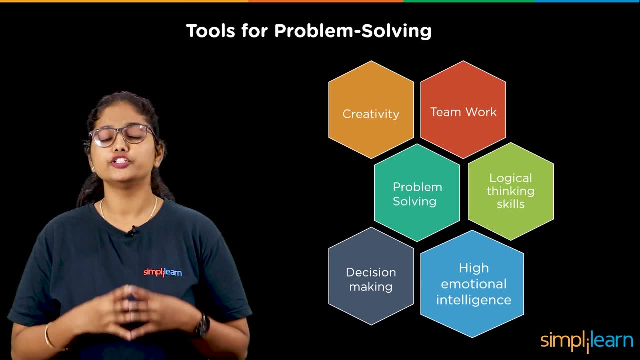 cause of problem and arrive at a best solution. you must possess analytical skills and follow a logical and systematic process. Next is a high emotional intelligence. You should have a high emotional intelligence when you are dealing with the interpersonal conflict problems. At last we 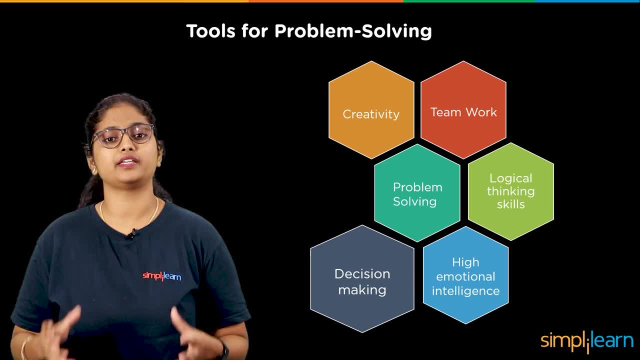 have a decision making. You should have a high emotional intelligence when you are dealing with the interpersonal conflict problems. At last we have a decision making. Problem solving and decision making go hand in hand. You must have enough confidence and faith in yourself to make a decision and see it through. 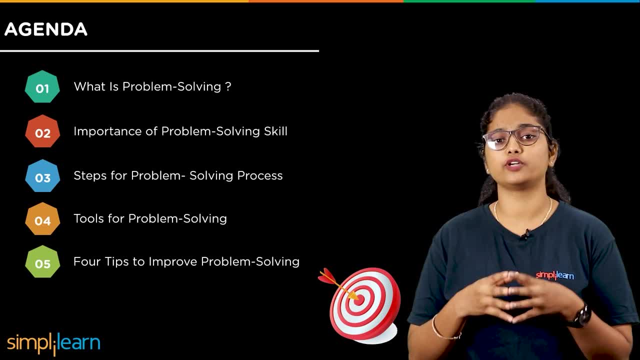 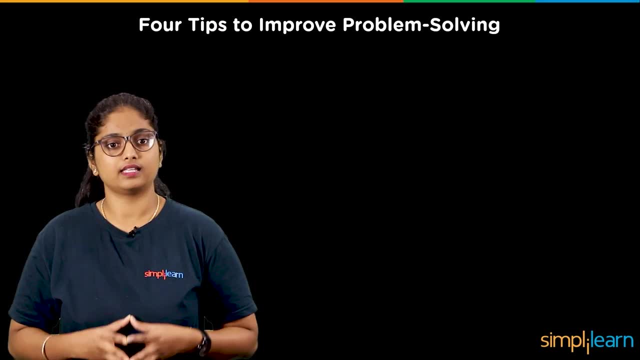 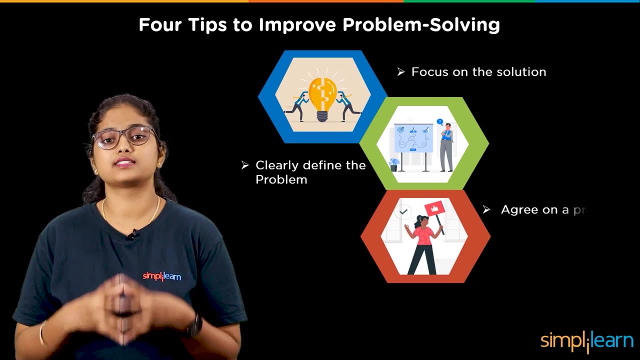 Well, now it's time to see some of the tips that helps to improve problem solving skills. If you feel uncomfortable when you're dealing with a major problem, don't worry, there are some tips to improve problem solving skills. Here are some tips that will help you enhance your problem solving skills when you're dealing with a. 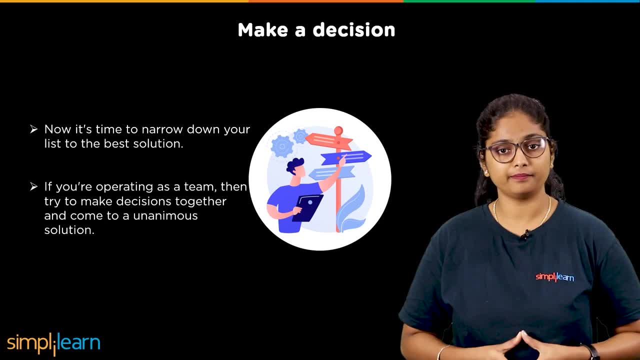 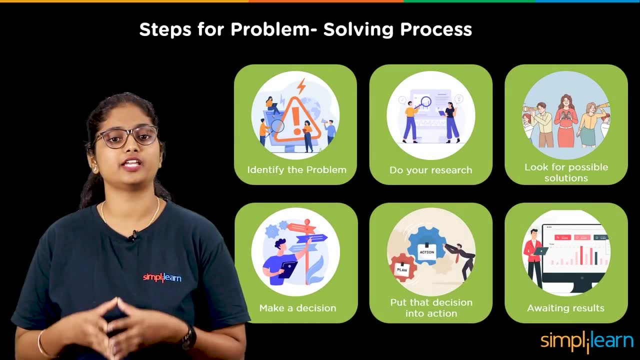 down your list into a best solution. If you're operating in a team, try to make a decision, to gather and come to an unanimous solution. The fifth step is to put the decision into an action. Implementing your selected solution is in a planned and calculated way will avoid the action. 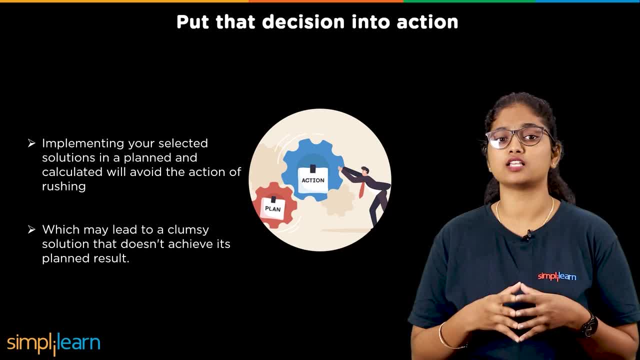 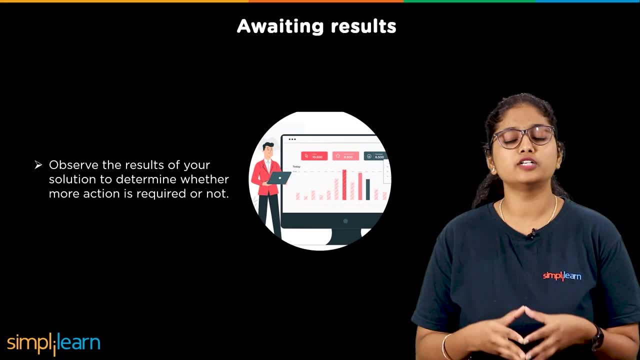 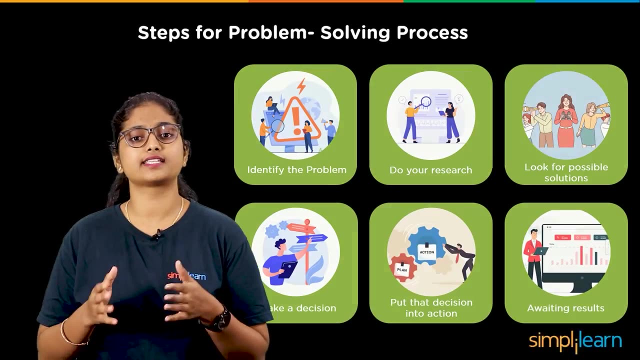 of rushing, which may also lead to a clumsy solution that does not achieve the planned result. And the last step is to awaiting for the results. Observe the results for your solution to determine whether the more action is required or not. Now let's see the skills or a tool. 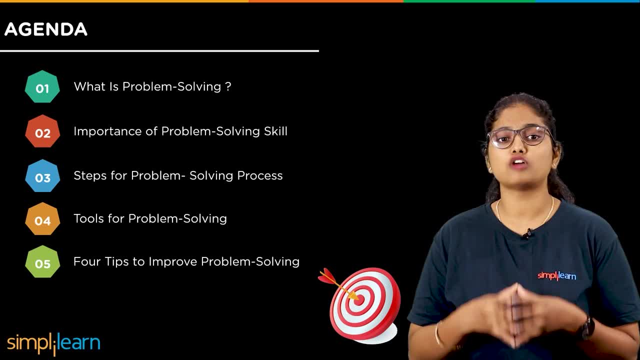 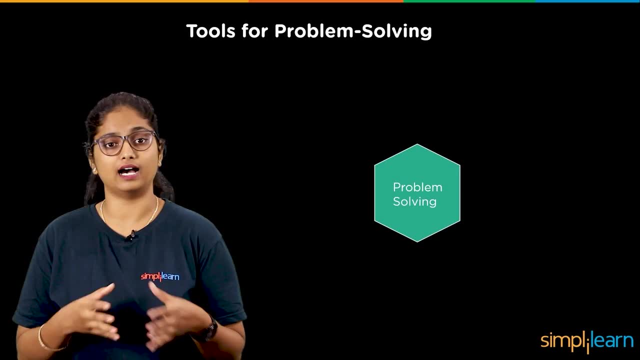 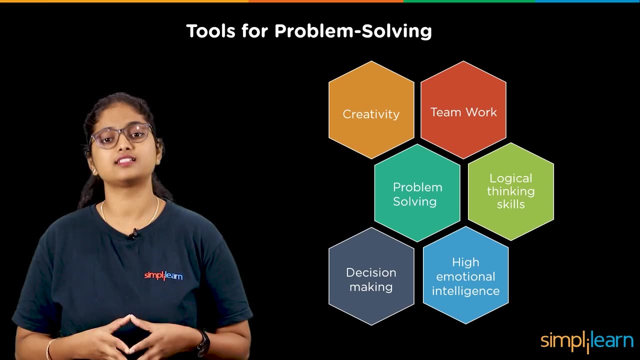 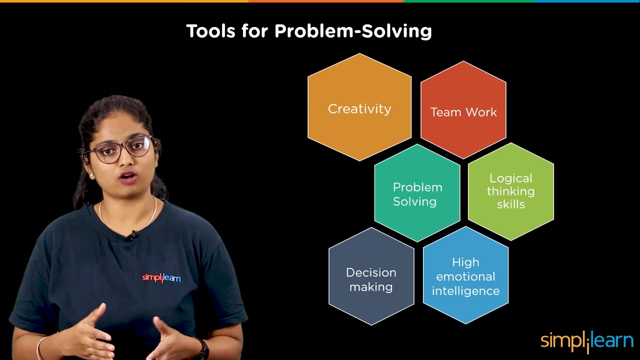 required for the problem solving. The best problem solver often have a few fundamental skills. The most important skills to draw upon when engaging a problem solving process are creativity, teamwork, logical thinking and high emotional intelligence and, at last, decision making. Let's see one by one: Creativity: Creativity helps to think outside the box and reach out the new. 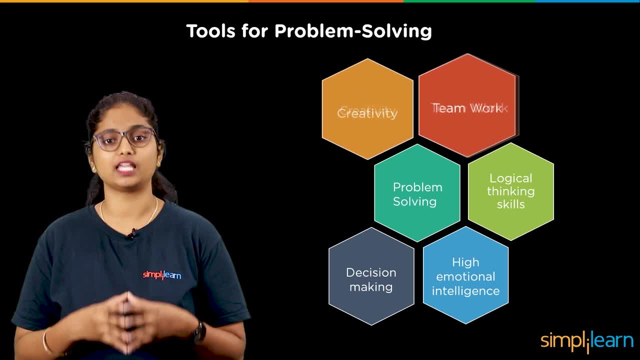 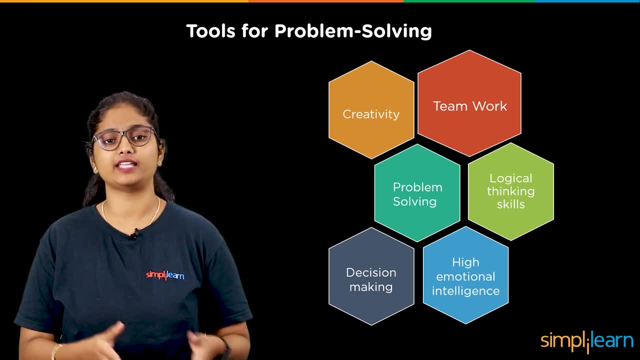 techniques and understand the problems. Next is a teamwork. Teamwork will help you address a group or a social problem, which requires working in a team collaboratively and supportively. On the list, we have a logical thinking skills To analyze the cause of problem and arrive at 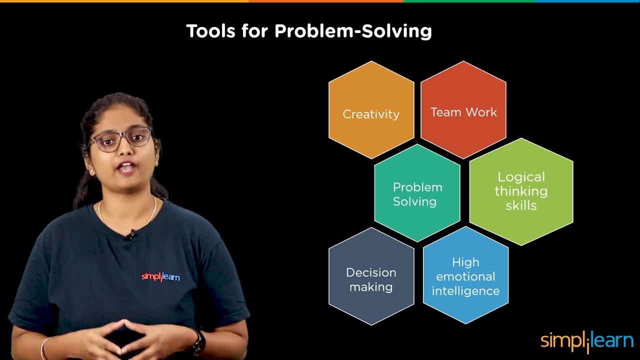 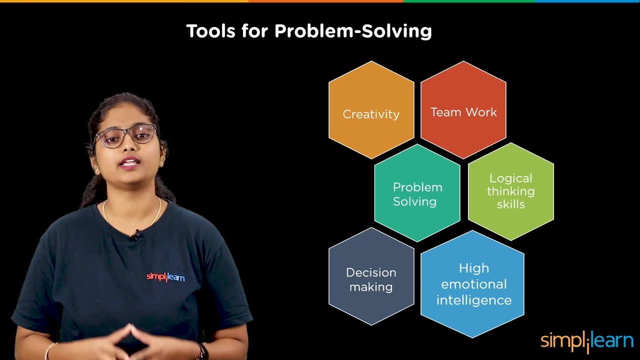 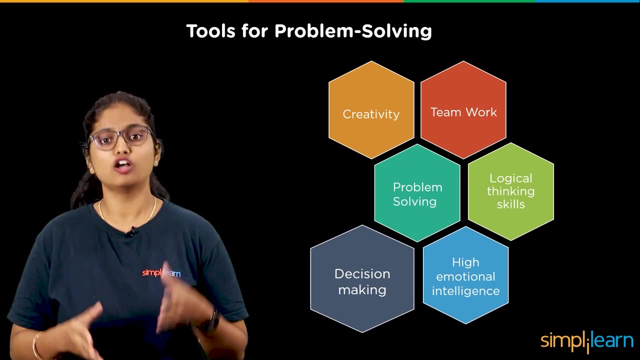 a best solution. you must possess analytical skills and follow a logical and systematic process. Next is a high emotional intelligence. You should have a high emotional intelligence when you're dealing with interpersonal conflict problems. At last, we have a decision making. Problem solving and decision making go hand in hand. You must have enough confidence and 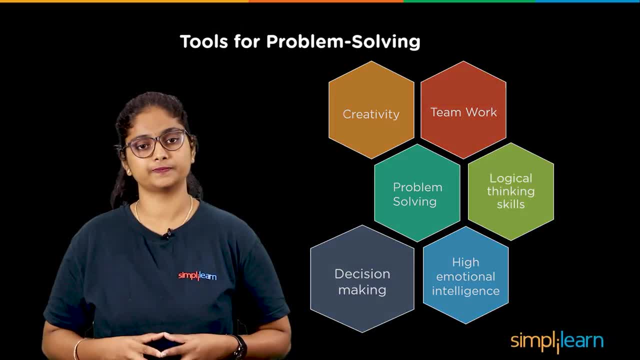 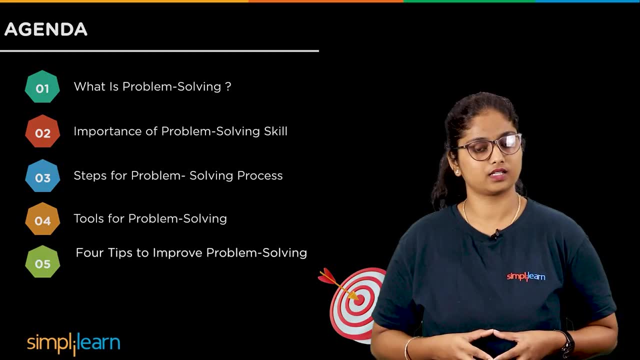 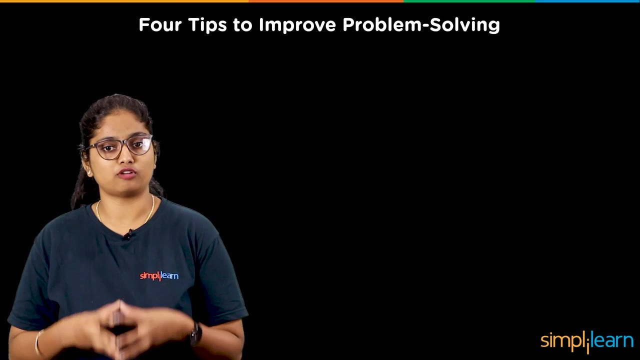 faith in yourself to make a decision and see it through Well. now it's time to see some of the tips that helps to improve your problem solving skills. If you feel uncomfortable when you're dealing with a major problem, don't worry. There are some tips to improve problem solving skills. 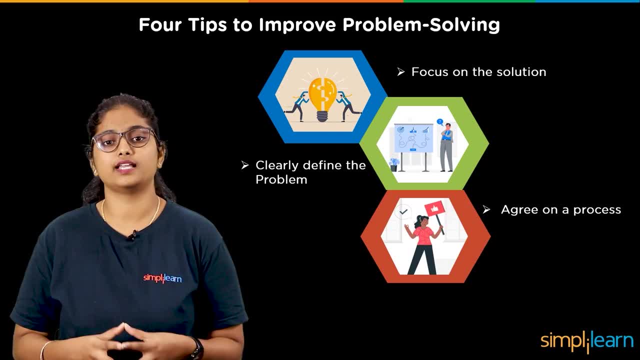 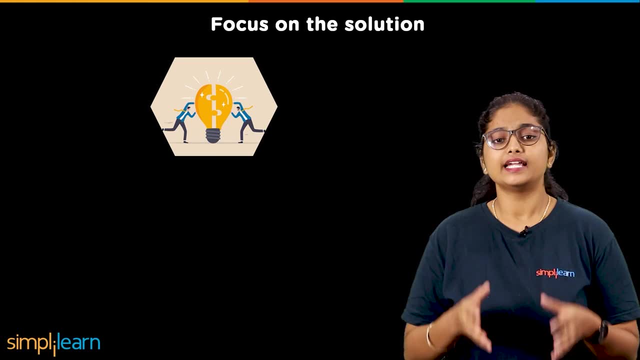 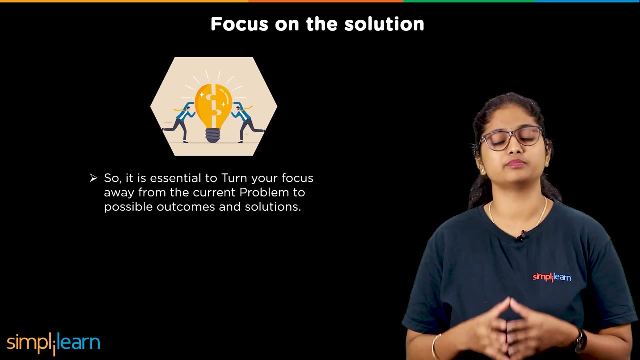 Here are some tips that will help you enhance your problem solving skills. when you're dealing with a problem Focusing on solutions, It's easy to become hyper-focused on the event that creates the problem, So it is essential to turn your focus away from the current problem to possible outcomes and solutions. This